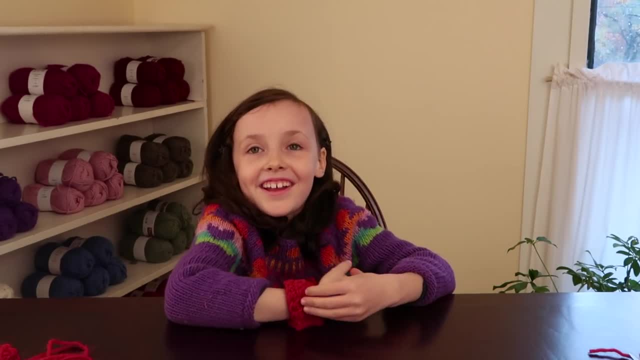 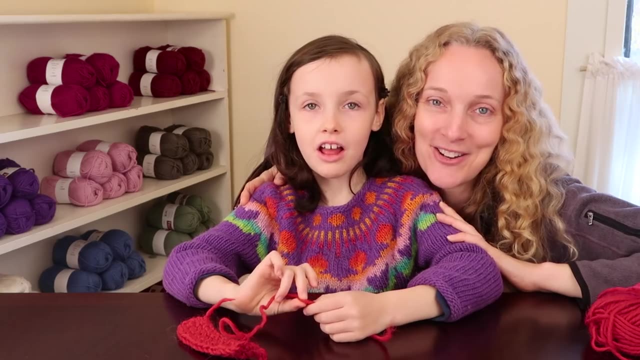 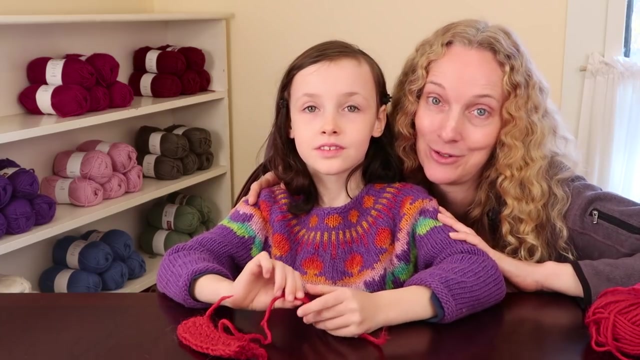 Today I'm going to show you how to make a kid's bracelet. Hi, this is Amy from Knitting Help, and with me today is my daughter, Erin. Erin is seven years old and she's been crocheting for a long time now. I think you were probably four years old. 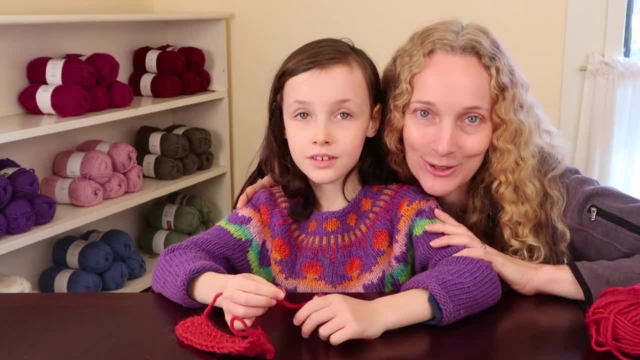 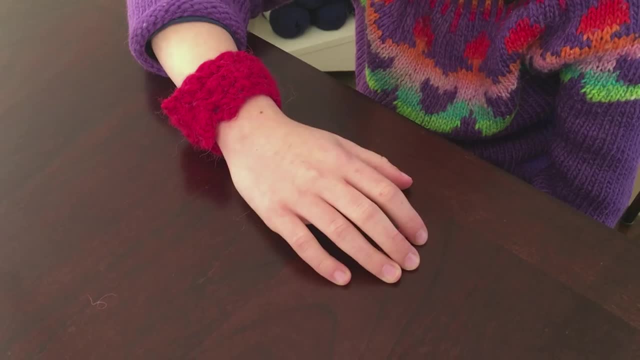 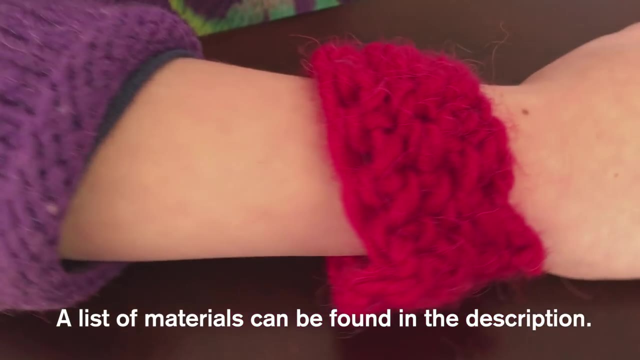 when you first started crocheting. She wants to show you how to crochet. So today, please welcome for the first time Erin Shalini Finley. What's the project you're going to be working and showing us today, Erin? This is a kid's bracelet. It can slip on and off easily. Great, And it stays. 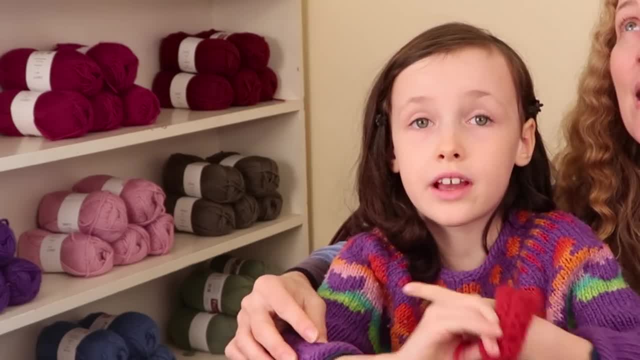 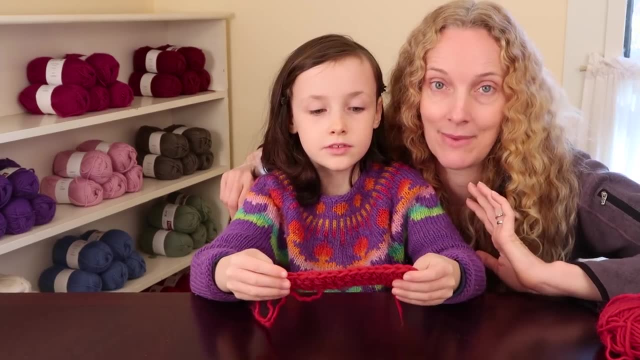 on. so if you're doing any gymnastics or anything, it will fall off. It's very fast to make. She's going to basically show you how to do a rectangle shape which you can make as big as you want and sew into whatever object you want. Okay, Erin, take it away. 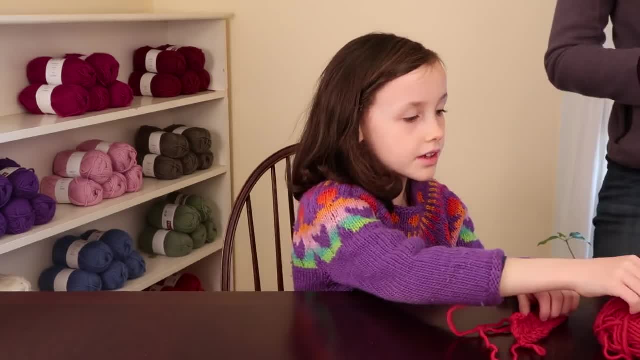 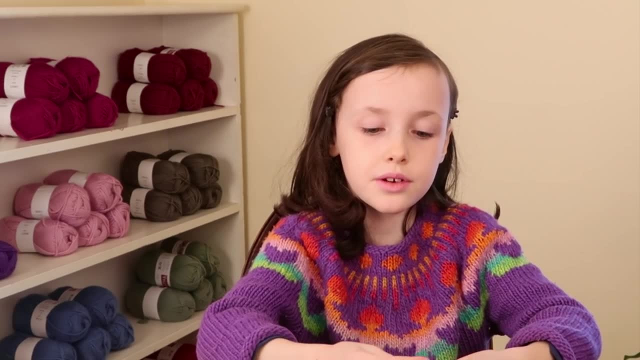 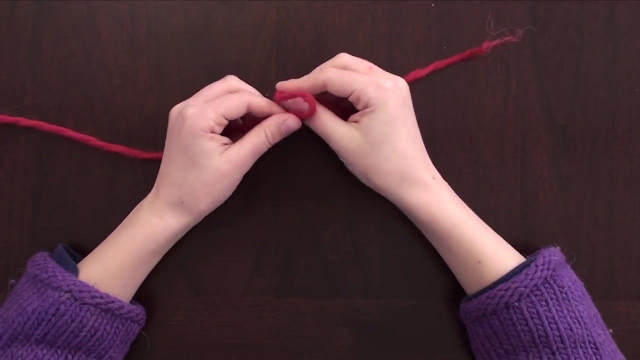 So the first thing you need, what you need to do um when you're starting crochet, is when you have to do a slip knot. There's two ways to do it, but I like to do it this way: You have to leave some um on the end of the yard for space and you make a loop. 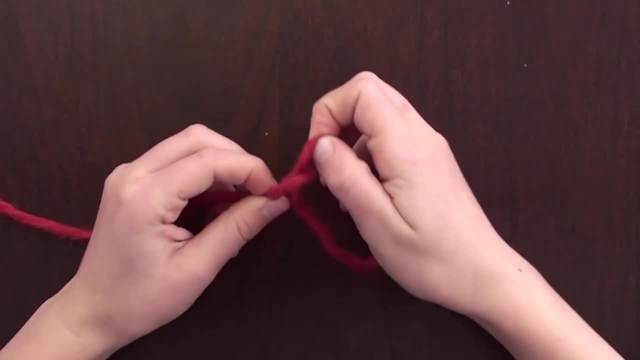 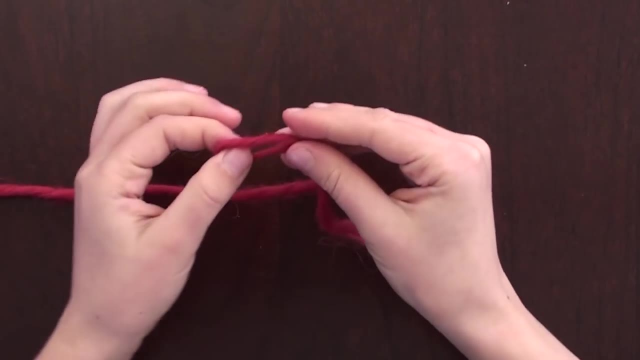 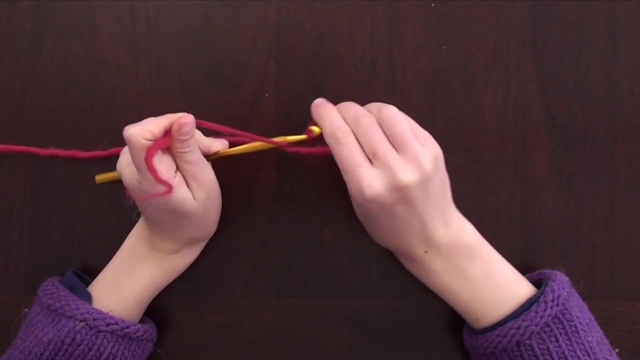 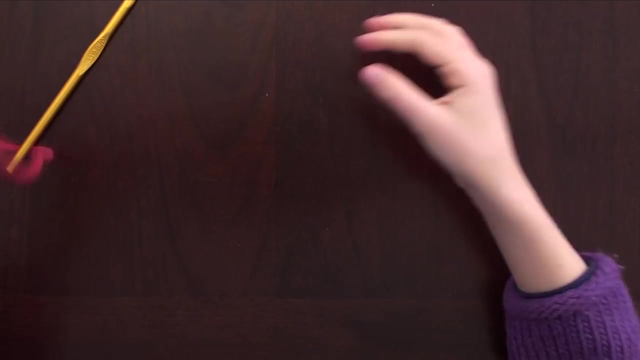 pitch it, make another loop, bring it through, then pull it, then pull the tail and this yard to make a slip knot, And then you can also put on the crochet hook and then you just pull both of them to tighten it, And if you want to get rid of it you just kind of yank it like this and then it just disappears. 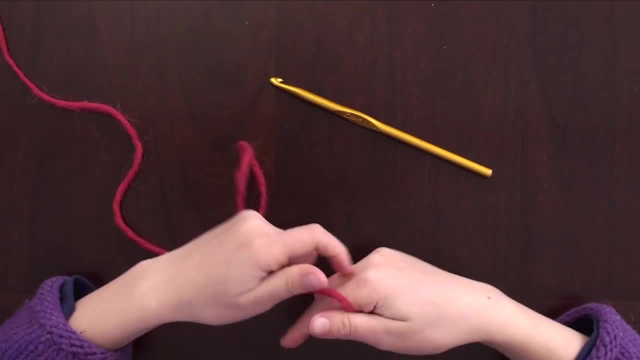 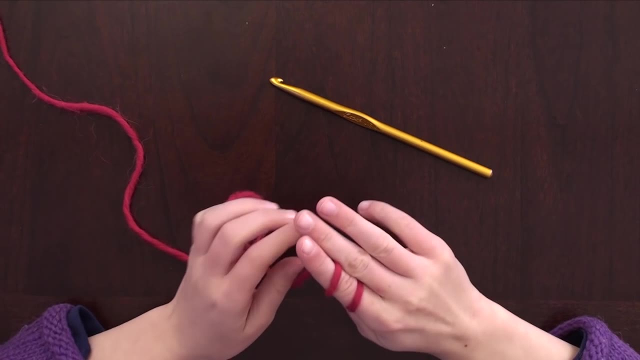 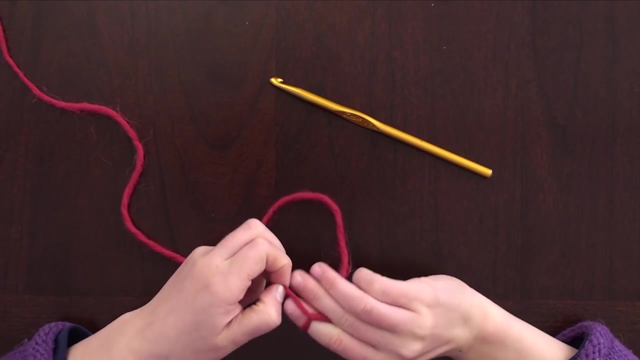 So the second way is you so you hold on to the tail like this and then you wrap it. you wrap it once, then wrap it twice. You pull this one almost over, almost over the your fingertip, then you pull this one over your fingertip, then you can tighten it at. 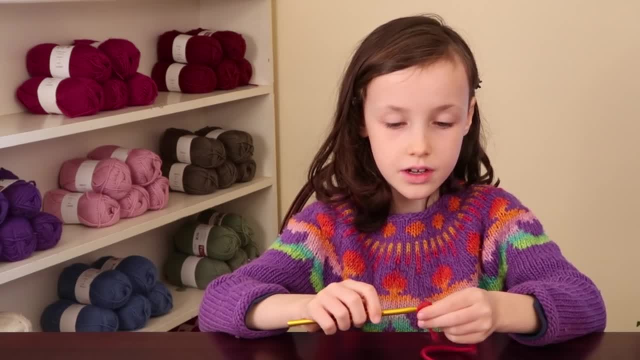 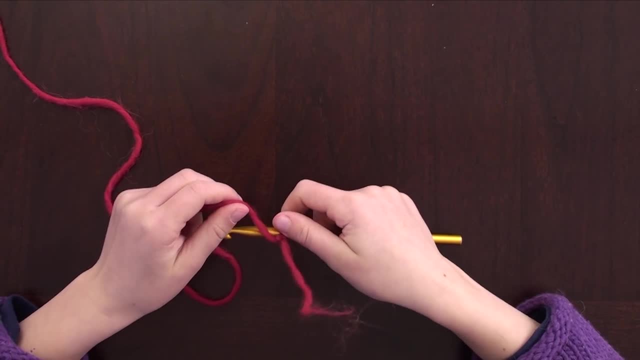 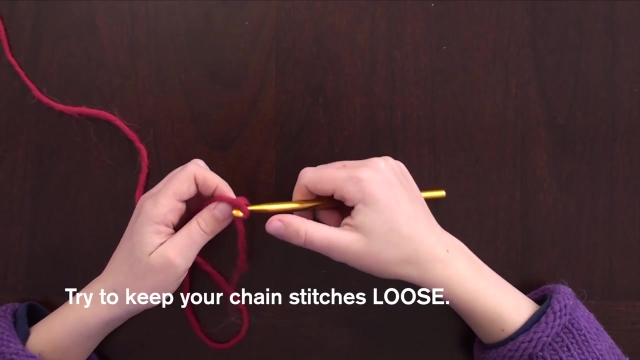 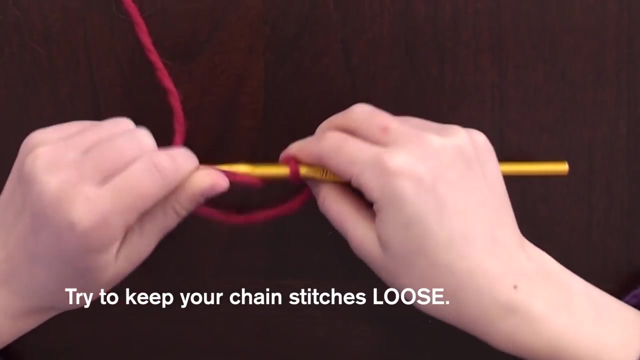 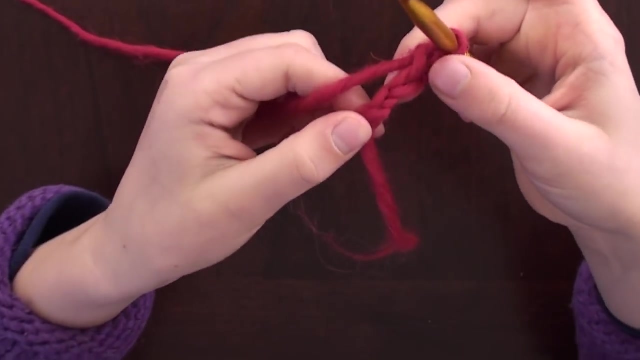 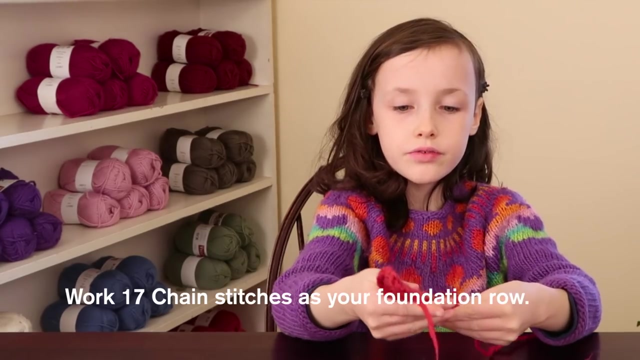 the bottom like this. Now I'm going to show you how to do the chain stitch. So how you do the chain stitch is you're you're wrapping around the hook, um, hooks it, then just pulls it through So you can see it kind of looks like a little little V's. So how you begin, begin the kids wrist. 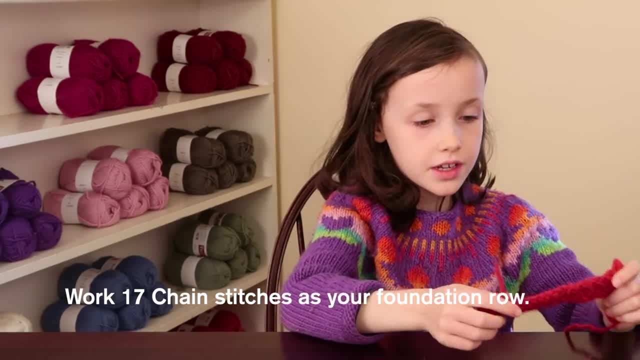 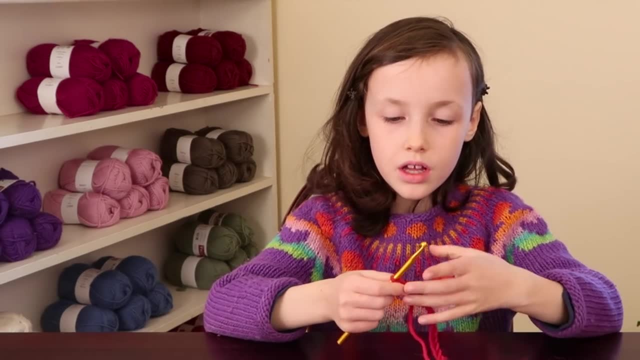 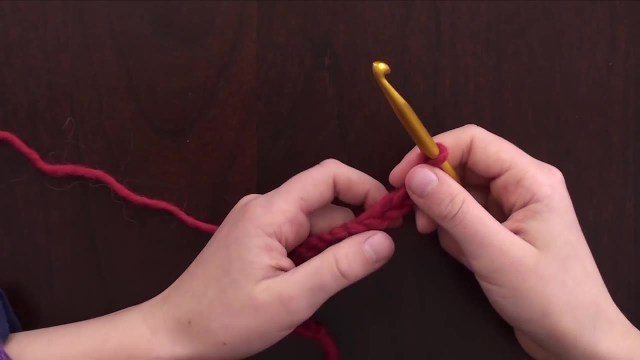 warmer. um, you start with, um, 17 stitches is what I did. At the beginning of the row of the row, you skip one of the V's. At the beginning of the row of the row, you skip one of the V's And then go on to the next. You're going, you're gonna go into the stitch, you're gonna go into here. 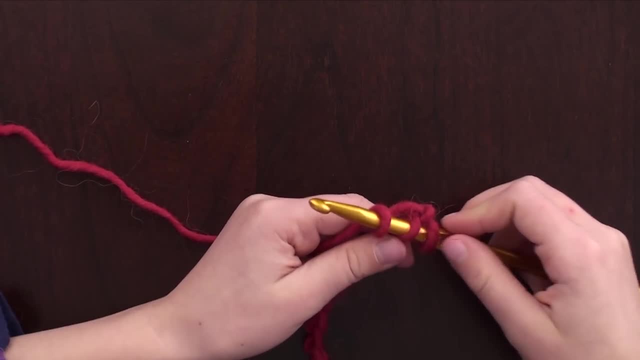 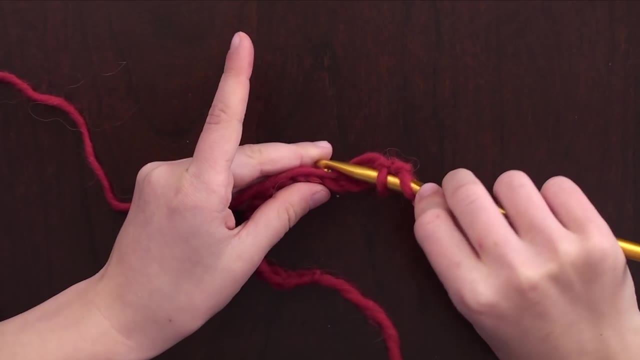 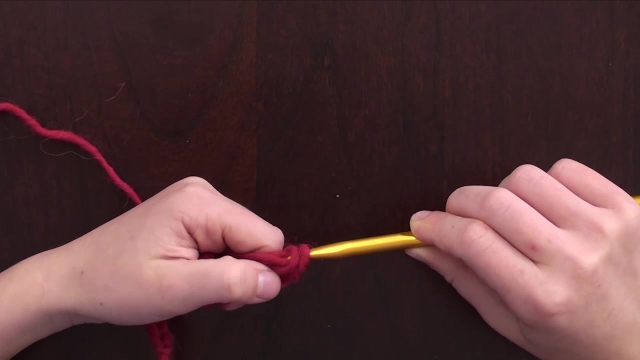 then grab, get the yarn, wrap it around once, pull, then pull it back. crochet of two loops: then you take this one and then you wrap it around, then crochet out like this And then you pull it through those two. Perfect, and that's one single crochet stitch. 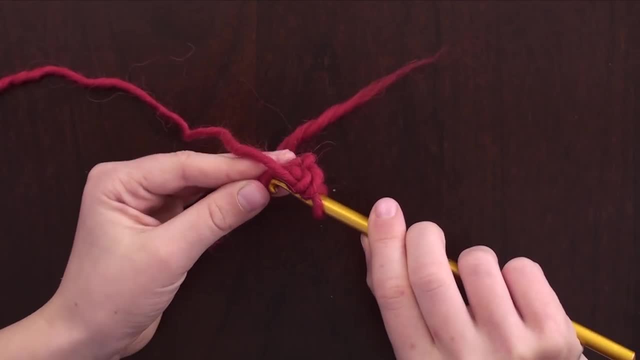 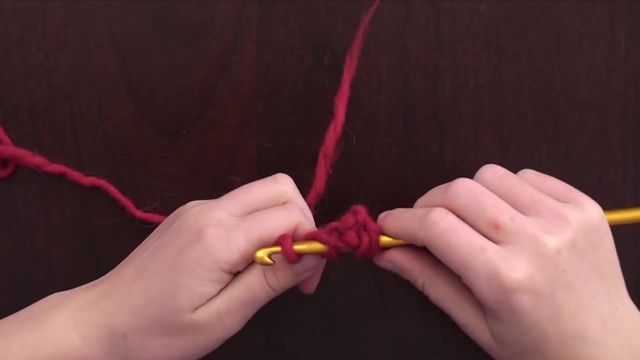 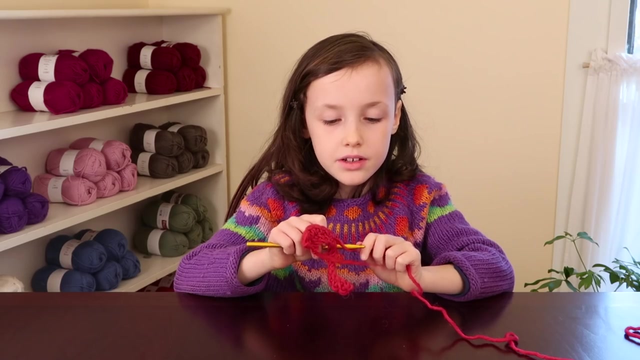 And now to do the next one, you go into the second loop. Yes, then you wrap it around. Now Erin's gonna tell you a rhyme she made up to help remember the steps of single crochet. Well, it's about a doggie. so the doggie goes in through the bushes. grab the bone. 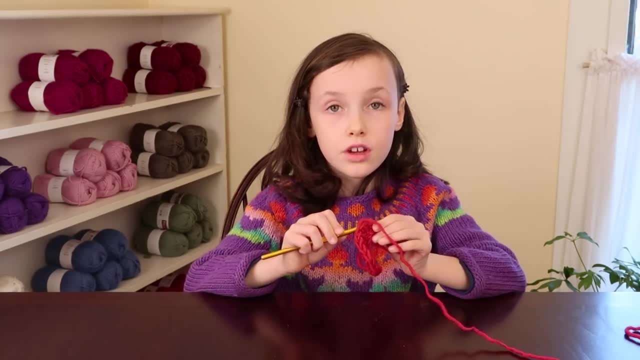 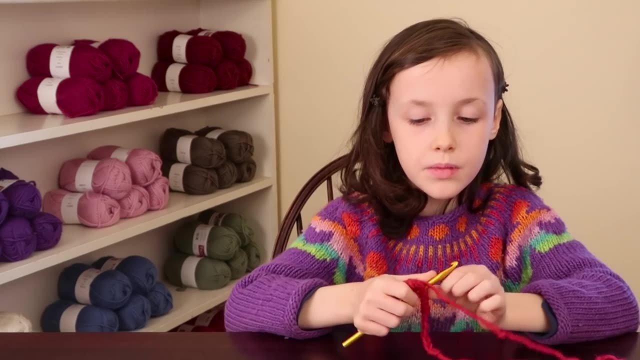 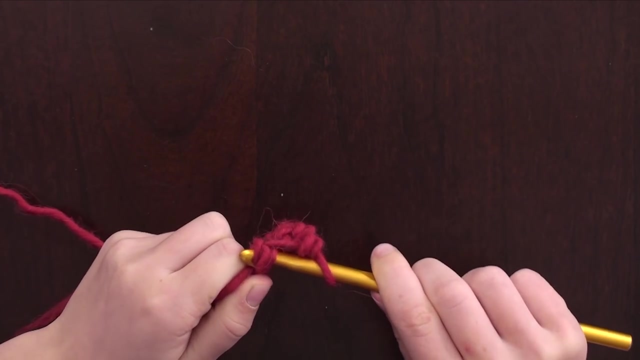 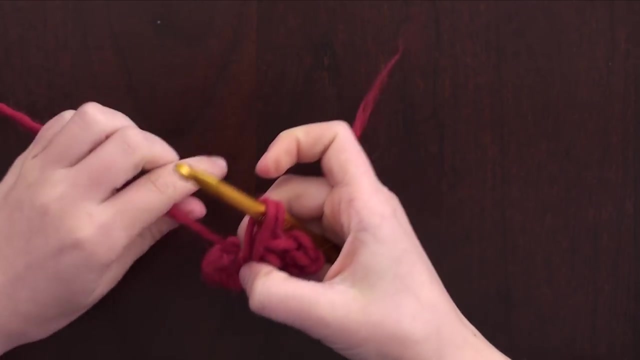 places through the woods right back home. So that's a term that you that will help you remember. And one mistake I sometimes do is I go through and then I accidentally wrap it like um two times. I can show you how to fix that. so it will look like this: You just get the top loop off and then you can tighten it like that. 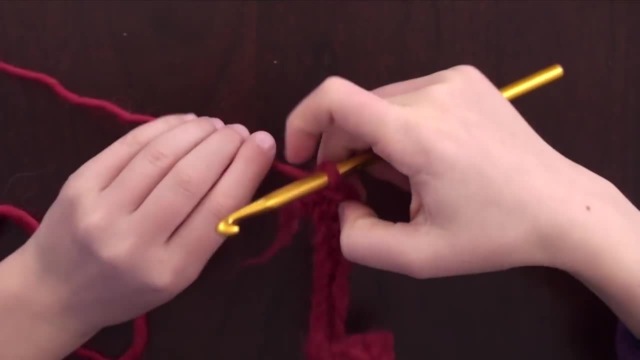 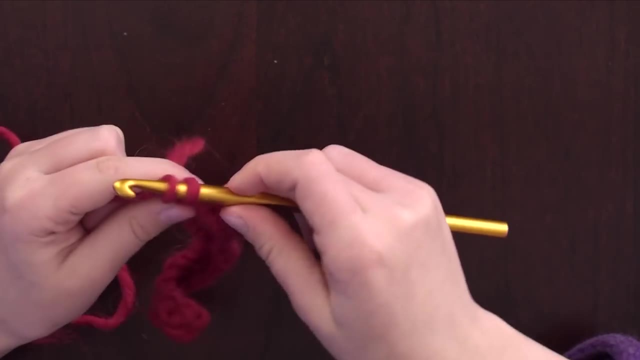 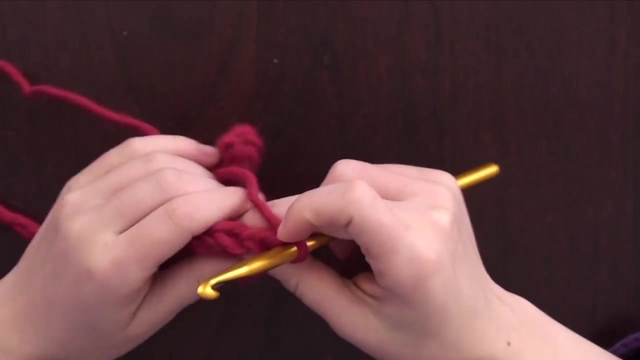 So I'm done with the row now and I'll show you how to turn around now. So what you do to turn around is you do one chain stitch like this. then you can just turn around The this yarn has to be in the back, not in the front, so you want to make sure it's at the back. 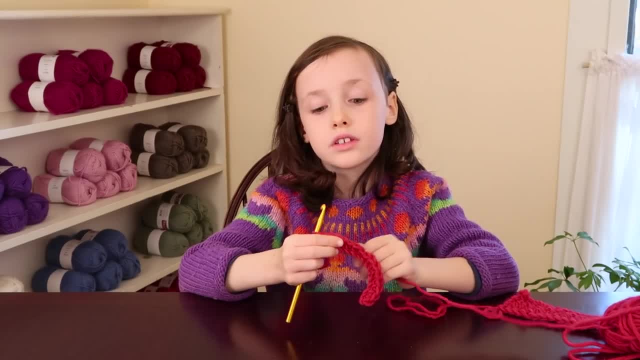 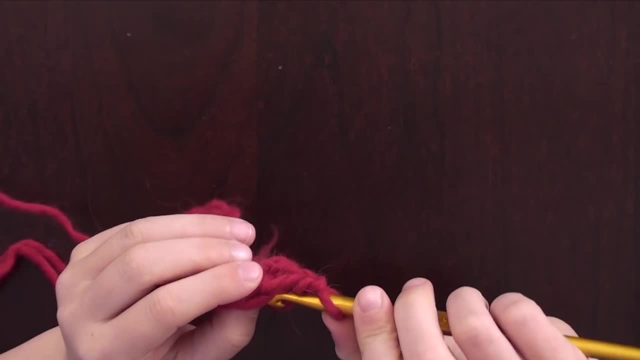 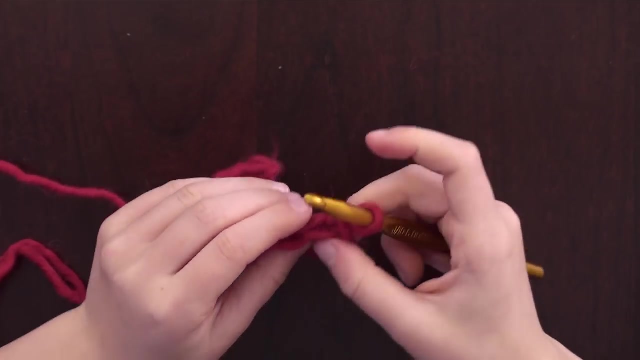 And now, when you work on your first row, you went into the hole like this: but now we're going to go to the chain like this: We're going to go under two strands, The entire. we're going to go under the entire heart-shaped. 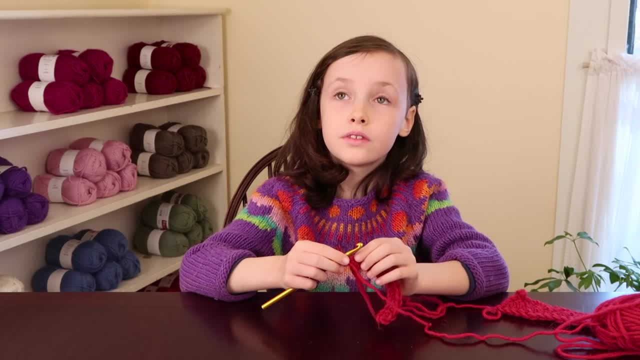 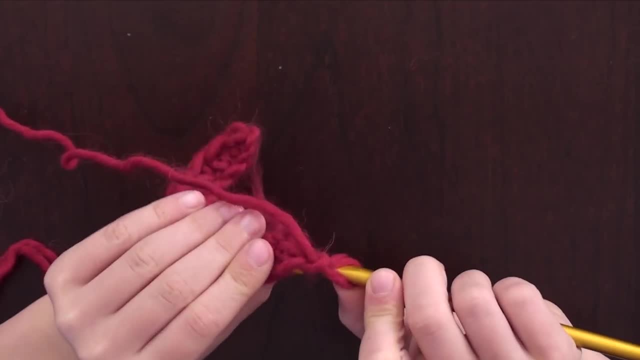 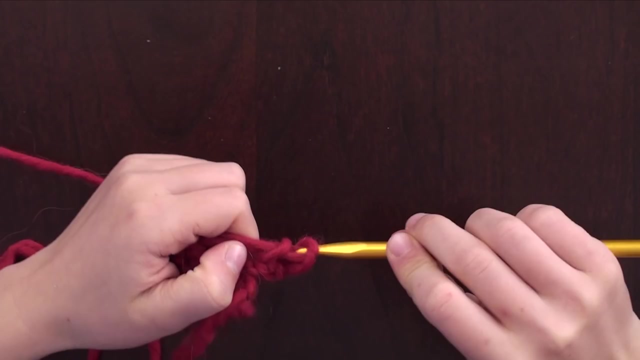 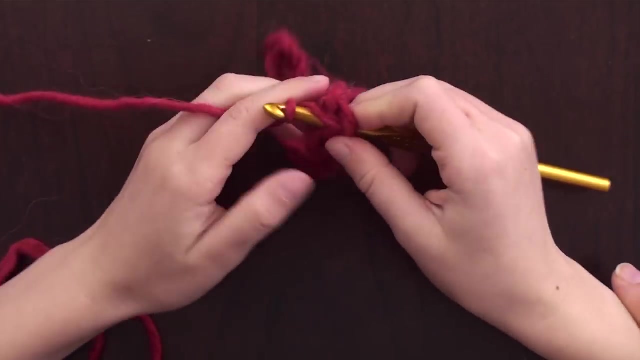 And remember to skip one, Or well, you're skipping just the chain. that you did, right? yeah, good, So you go into here. you just do the same thing. You do the same thing as you did on the first row, So you do four of these and that's how you make a kids bracelet. 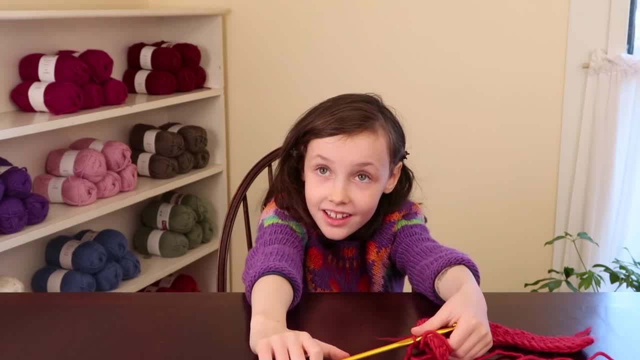 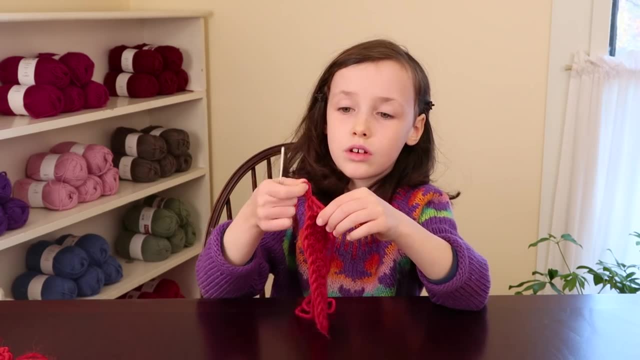 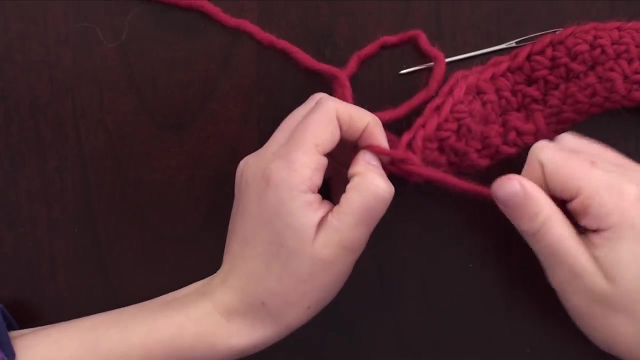 All right, four rows of single crochet, and then can you tell us how to stop the crochet? So, um, how you end it is: you get it off the crochet. you, you know, see the slope. so you get, you get this yarn, then you trim, And then you pull it right through and then just give it a little tug to tighten it. 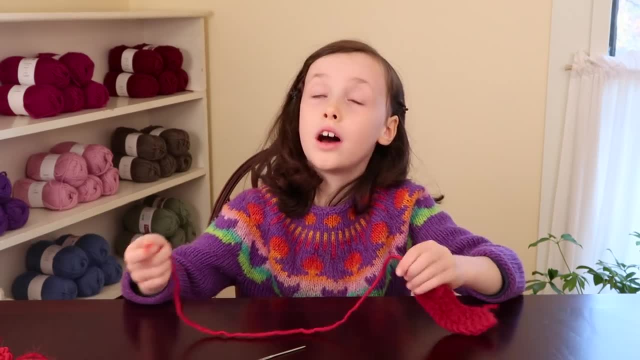 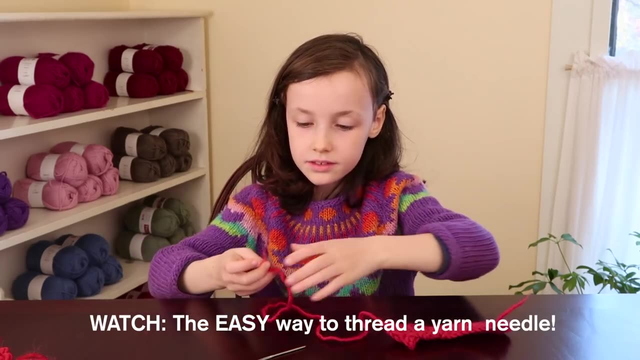 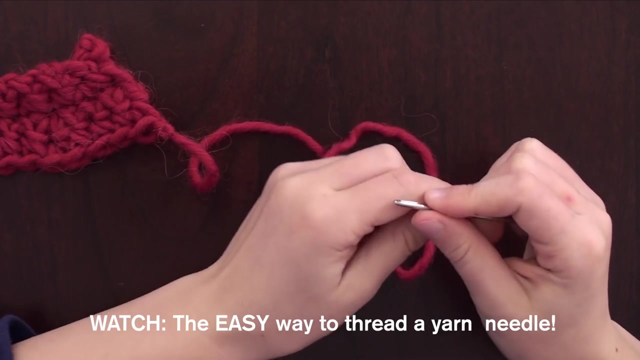 And you have to have, um, at least the foot of your yarn left. So now we're going to show you sewing. So a trick that I learned is you make a little like a loop like this, Pinch it as tight, as nice as you can, then just slide it off. 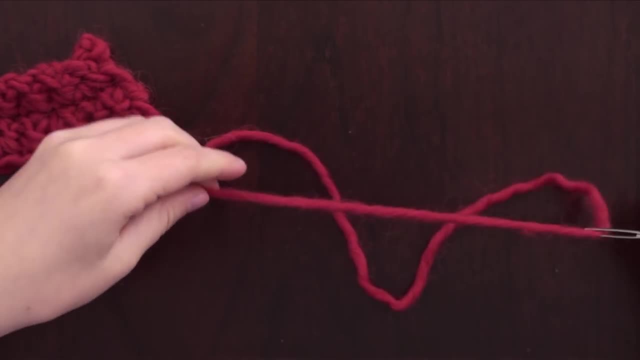 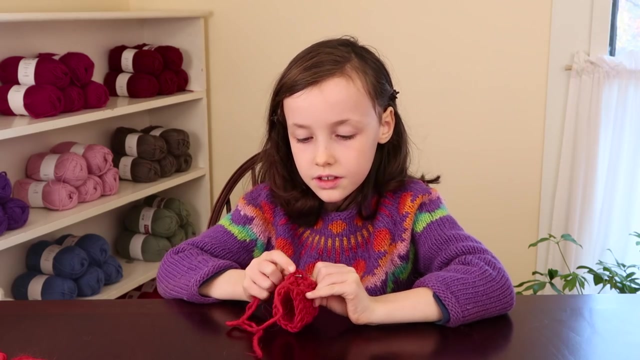 Then hold it tight, then you can just get it through the needle easily. You don't have to tie it, you just leave it like this. Now you do this, So you're going in through here. You don't want to get the tail stuck in here there.